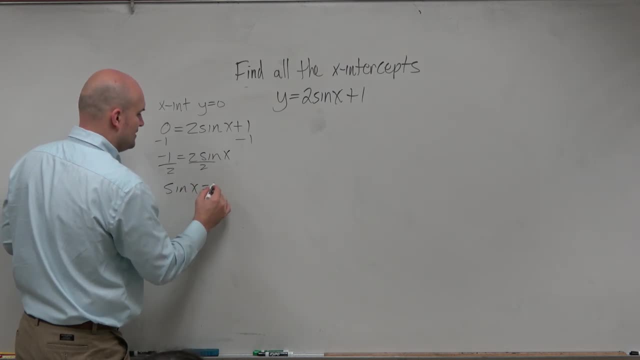 I want to solve. if I want to undo the sine. I know how to undo multiplication by division. I don't know how to do that right now, right, So I'm going to come back to this. But at this point some of you might have been like, hmm, I don't know how to undo sine, So let's. 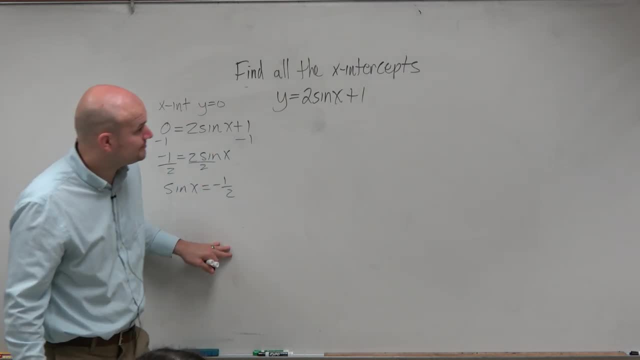 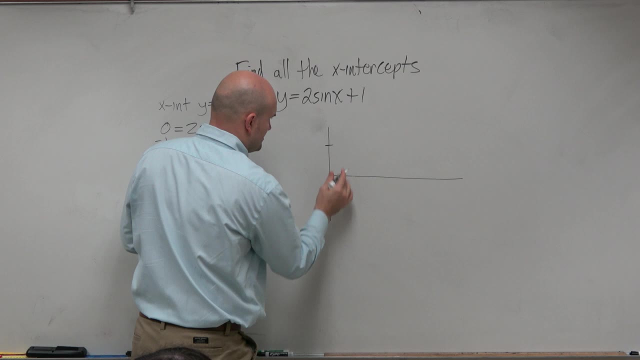 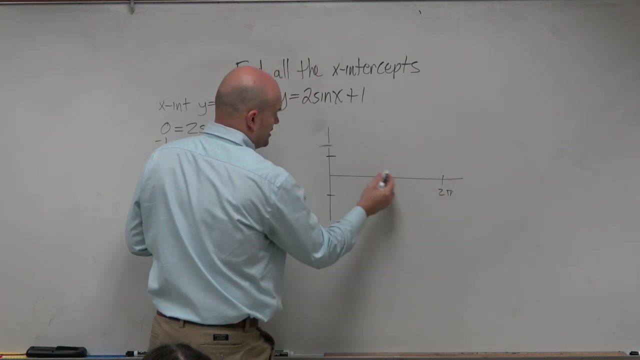 go and take a look at the graphical approach and then we'll come back to this. all right, So the graphical approach. well, we know that the sine graph, at least the initial period, goes up to one, downs to negative one and repeats at two pi. So I'm going to cross to. 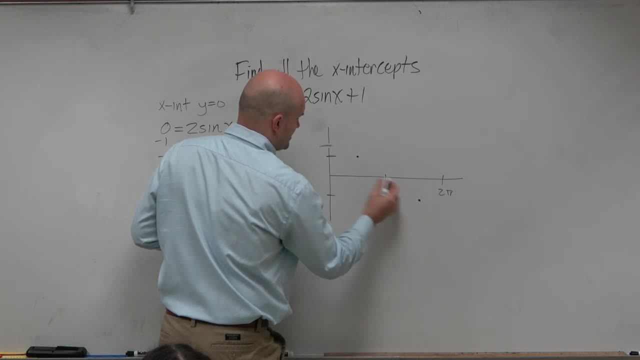 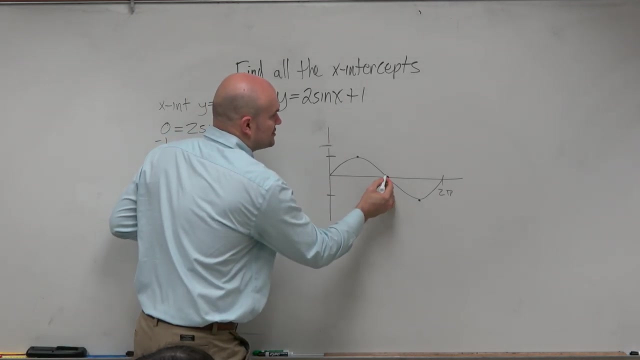 that pi. So this graph, It's going to look something like this, right? And if you're like, hmm, I can't really remember exactly, well, again guys, just go back to your unit circle right, Here's your coordinate. 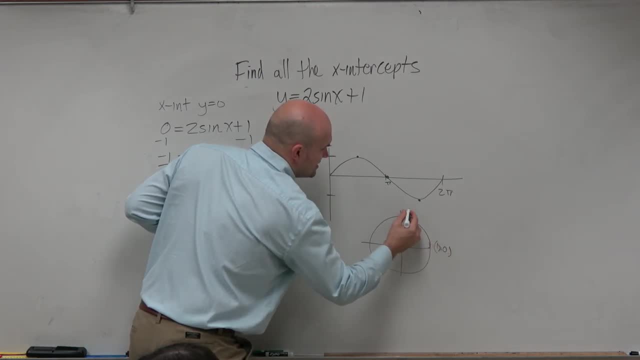 points. Sorry, one comma zero, Remember. sine is the y-coordinate, So that's zero comma one, This one's negative. one comma zero. And this one is zero comma, negative one. So at zero degrees the sine is zero. At pi halves the sine is one. 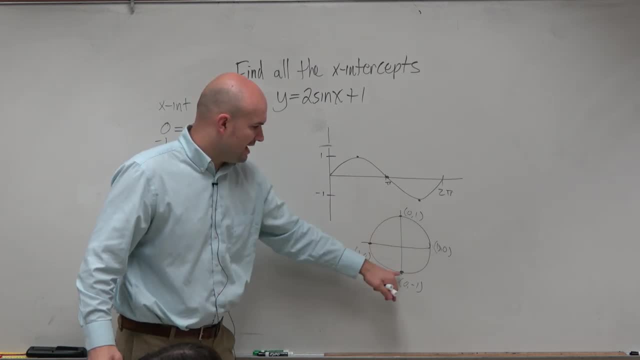 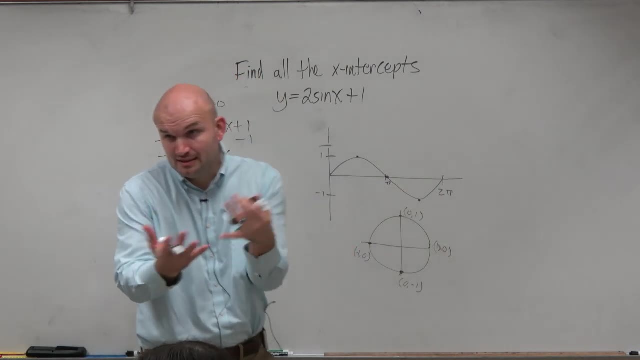 At pi the sine is zero. At three pi halves the sine is negative one, And then at two pi the sine is zero, right? So we can kind of quickly come up at least with that graph, in case we just forgot it, right, If we forget what the sine graph looks like, it's on a. 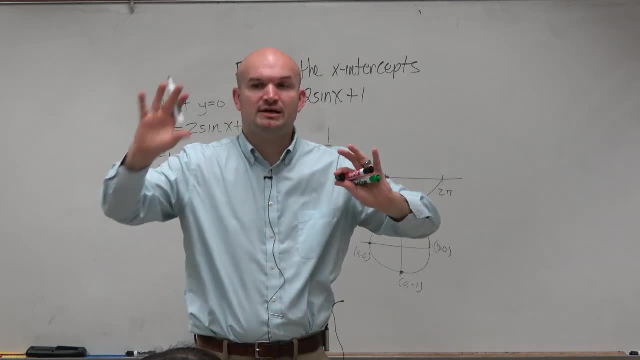 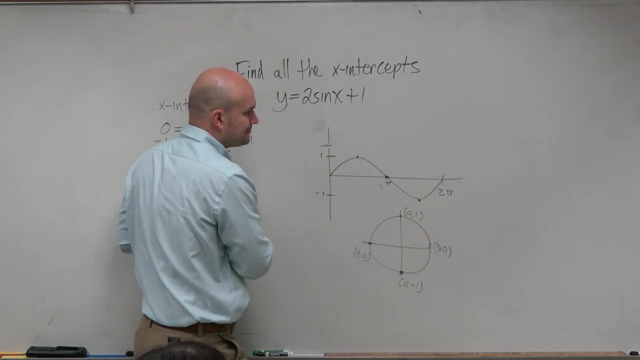 task. we're like, oh crap, We can just go back to the basic unit circle and evaluate for sine and do that. That's what we did that first day. You don't need to do all the points to get a rough sketch, all right. And then we look at this. We say, oh OK, so what is? 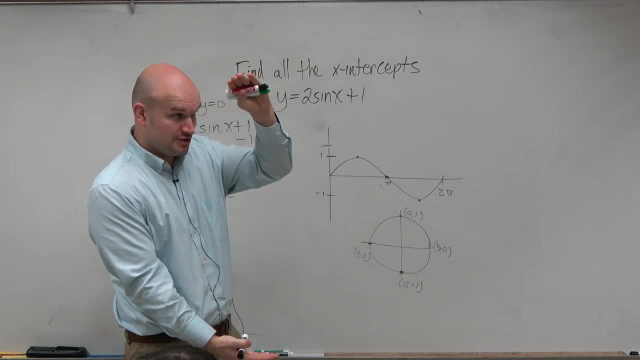 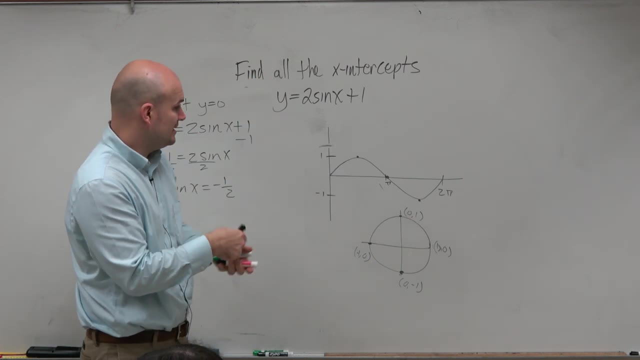 this doing? Well, that's stretching it right. The amplitude is two to two, So now it's going to go down from negative two to positive two. The range would be negative two to two, But then the graph gets shifted up one, So now it's going to go from negative one to three. 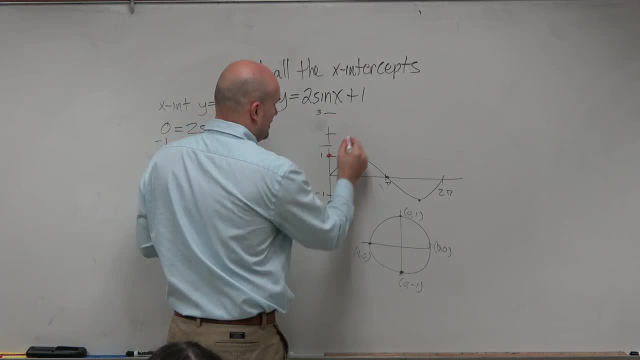 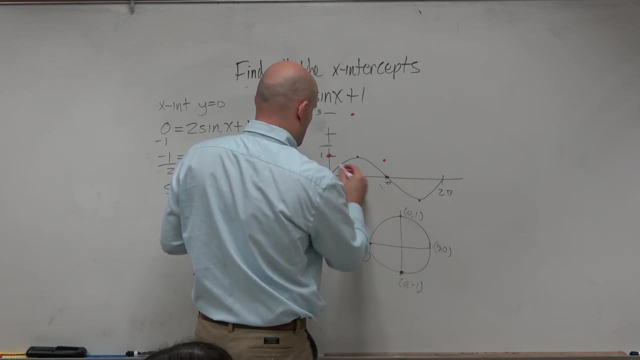 So now the graph kind of starts here And it's going to go up and go down. Let's see It's going to cross from there And then it's going to go up to two, then down to negative one. So it's going to share that point And then it's going to come up to there. So now 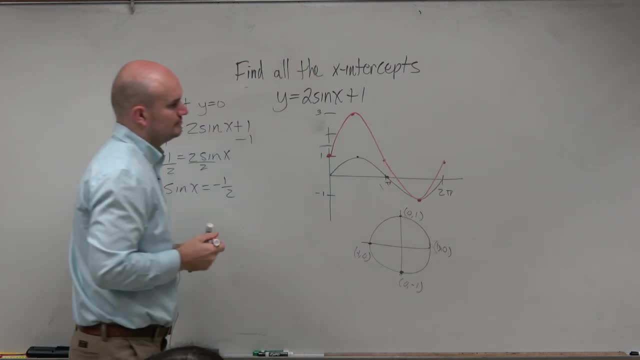 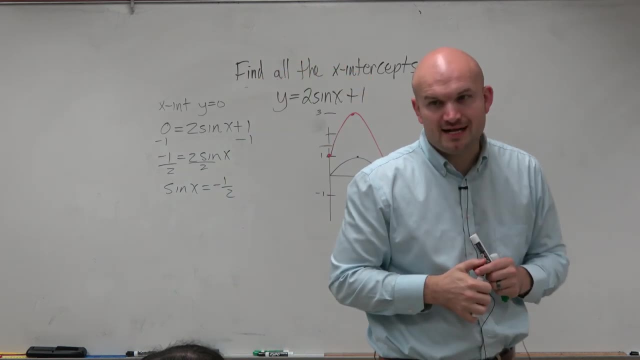 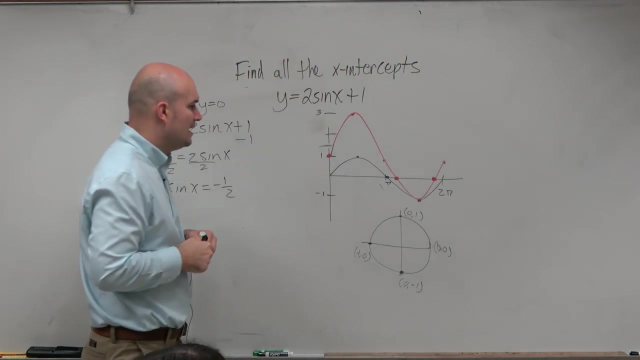 the graph looks like this: So now we know, here's the points. But crap, I don't know what exactly those values are. right, I don't know what those values are. So if we go ahead and take a look at this, so the graph doesn't help us out really. 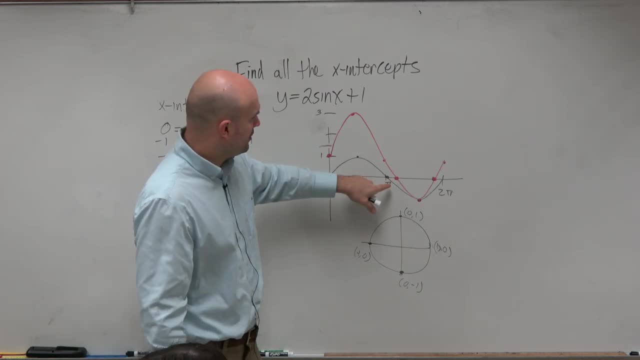 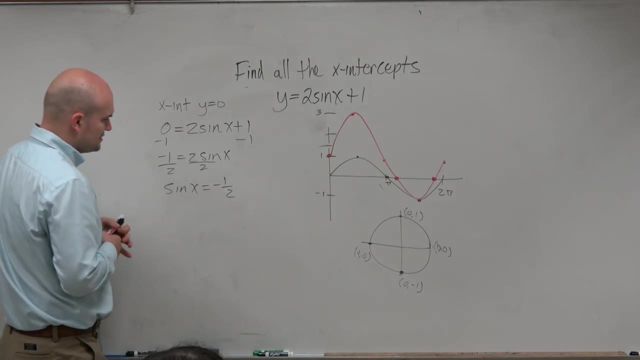 like the rough sketch. But we can kind of see these points are close to pi and close to 2 pi And that's kind of interesting And we'll come back to that. So let's kind of go back to this idea, all right, So we have the sine of something equals. 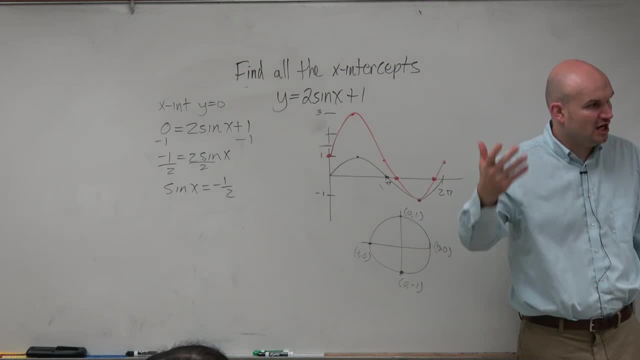 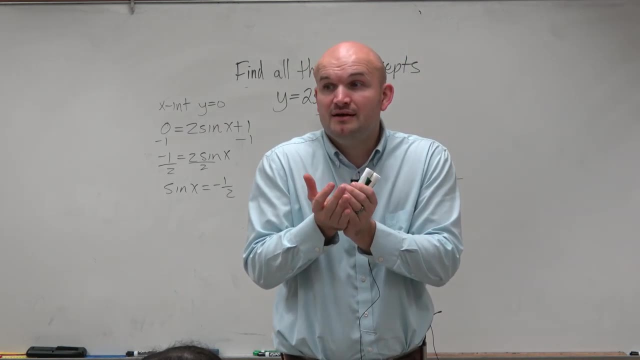 negative 1 f. So then I start to think to myself: what do I take the sine of? What does the sine function mean? Where do we include the sine function? We always take the sine cosine tangent of: Well, let's go back and look. Remember guys, Remember the good old. 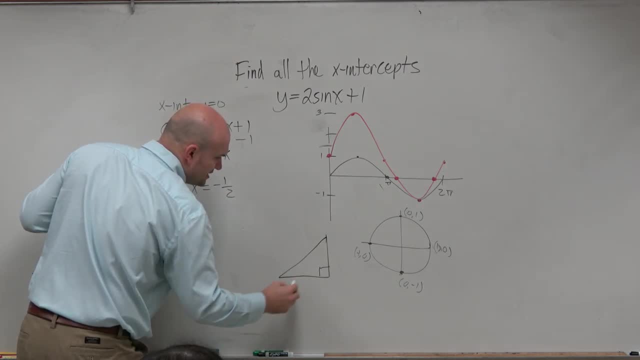 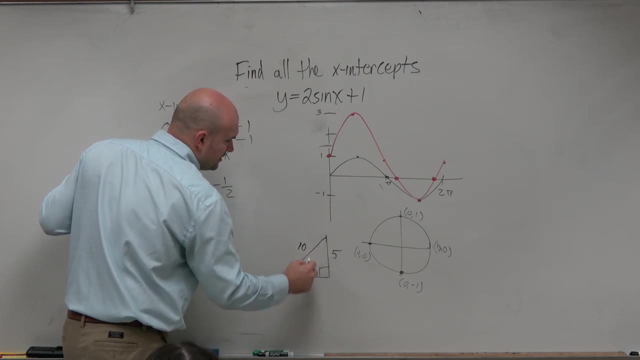 triangle days, Probably like man. why can't we just do like sine cosine tangent of like triangles? If I had like 30 degrees, 30 degrees, 30 degrees, And I said this was like 5, 10,, 5 square root of 3. If I was going to take 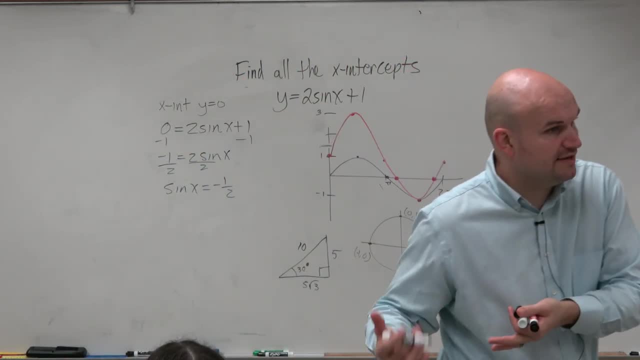 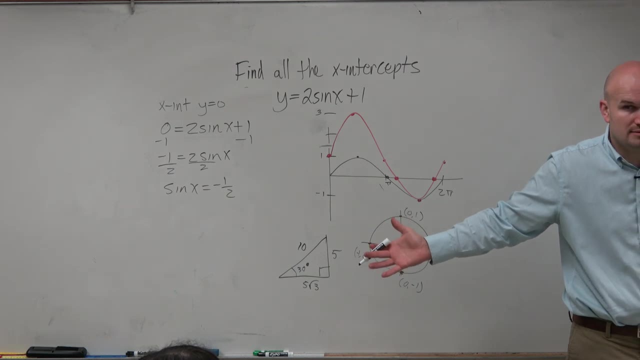 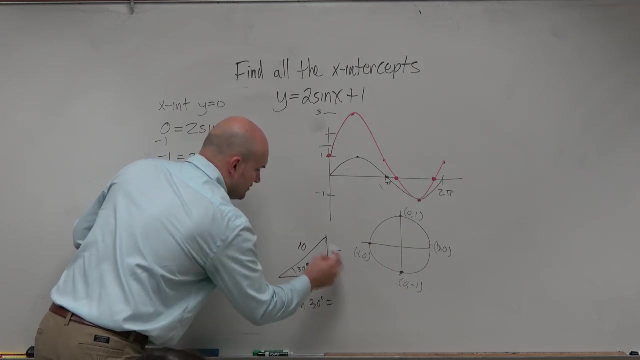 the sine. what would I take the sine of? If I was going to represent, if I was going to write the sine function here, how would I do that? Yes, Just what would I write? Sine what? 30. Sine of 30 degrees. So I'd say sine of 30 degrees is equal to 5 over 10, right, I can. 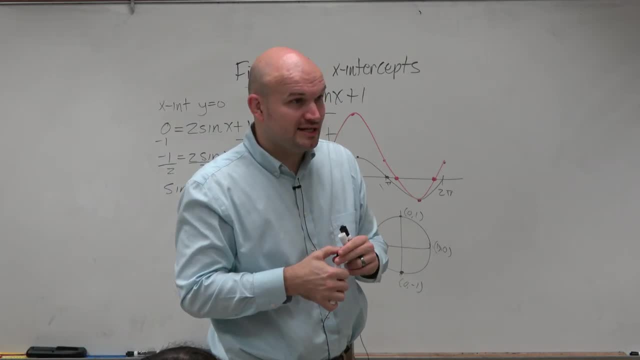 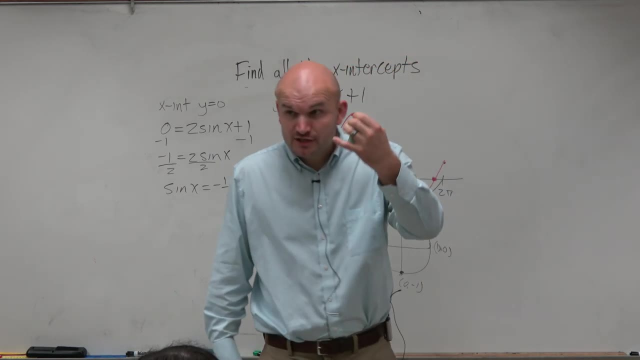 write that equation based on that triangle. But there's another thing that I'm trying to do with this, or I want you guys to understand. I'm taking the sine of the. what Angle right You take, trigonometric functions are based. 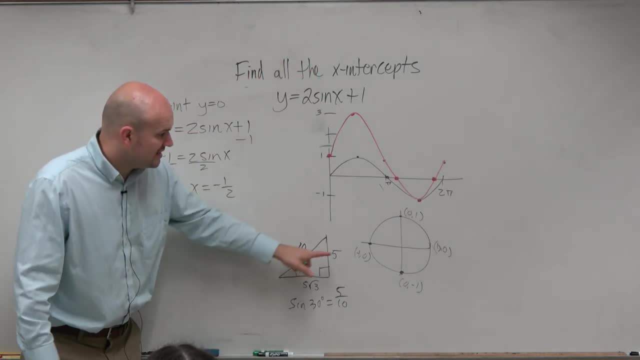 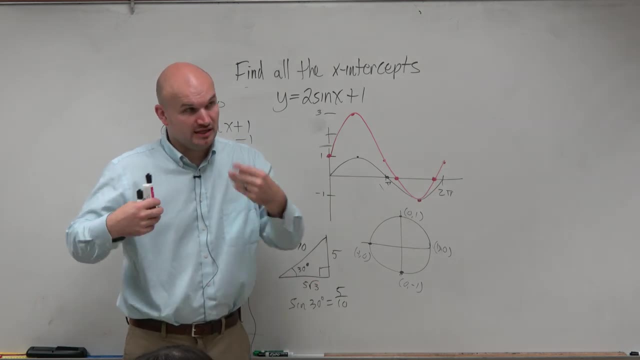 on the angle. It's the sine of 30 degrees opposite, over hypotenuse Right. The sine of an angle represents the ratio of that triangle. We have just been the last couple of days, we've just been so focused on the unit circle. But remember it's the trigonometric functions. 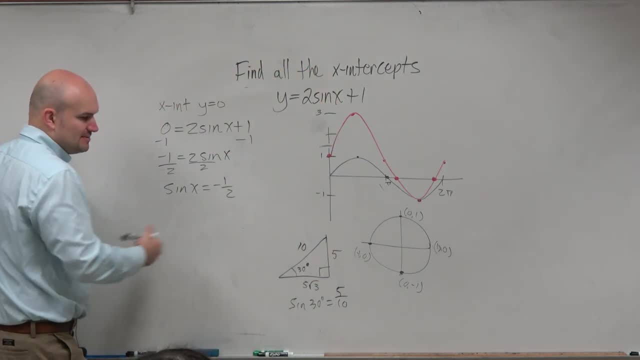 of an angle. So that's important. 30. say like sine of 5. No, that 5 is a side length right. The sine represents that ratio, correct? Somebody follow me on this? So when I look here it's saying the sine of what angle? 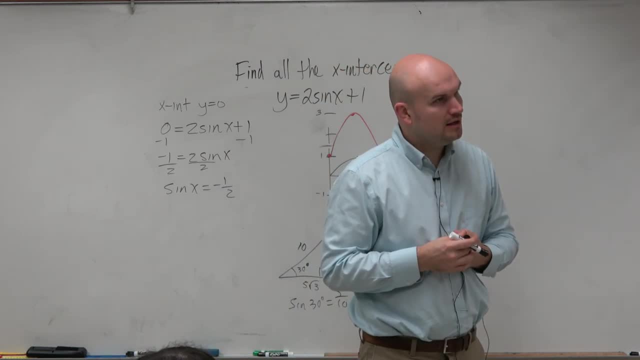 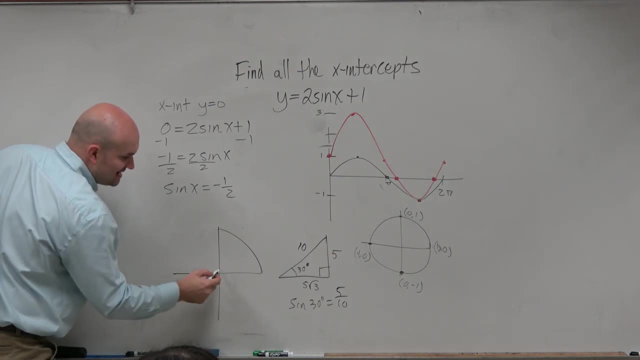 equals negative 1 half. And then I say, oh OK, well, I know, Let's go back and think of the unit circle now. So I know the sine is equal to 1 half, positive 1 half at square root of 3 over 2 comma 1 half. 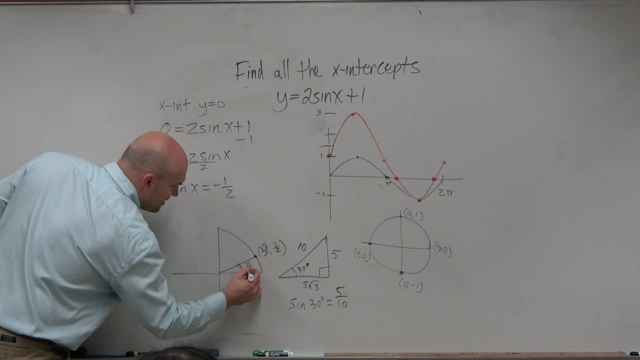 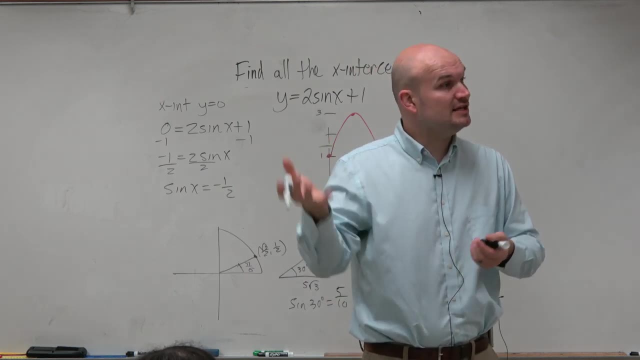 At this angle, which is since I know my first quadrant of the unit circle is pi over 6. Everybody agree with me. So now I've got to think: well, when is sine going to be negative? And I say, well, sine is negative in the third. 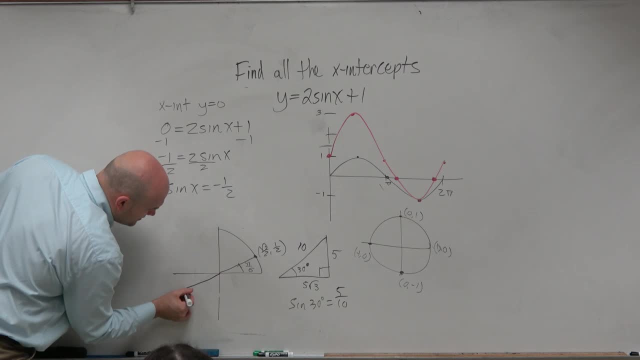 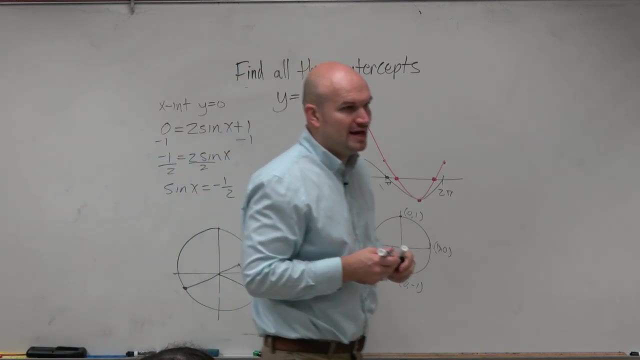 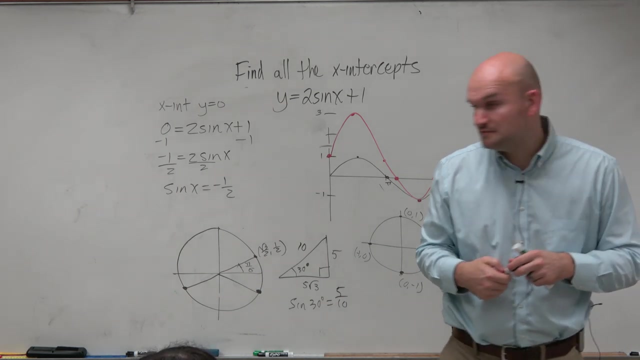 and the fourth quadrants. So it's going to be that reflection down here and down here. So now I've got to think: well, what angle then gives me negative 1? What angle then is going to give me negative 1 half? 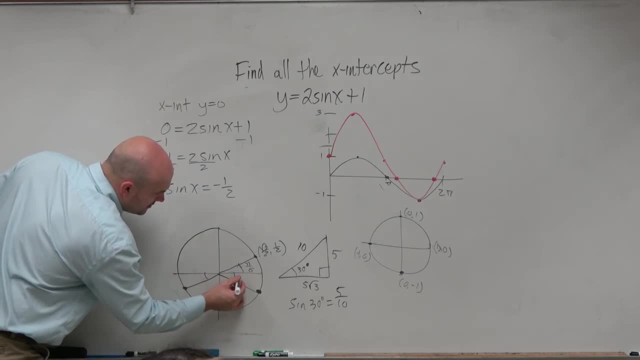 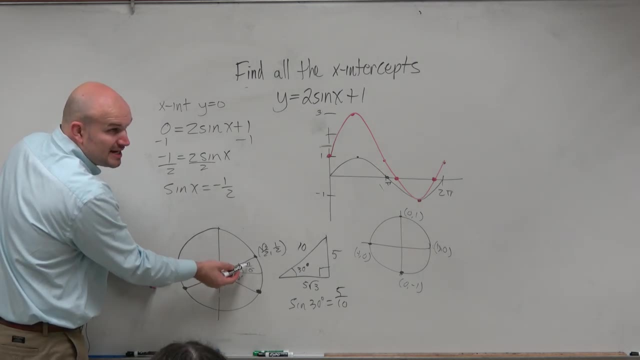 Remember they all have the same reference angle, right? So this angle is pi over 6 away from the x-axis, This one's pi over 6 away from the x-axis. So if I was going to say halfway around a circle would be pi in terms of 6, would be 6, pi over 6.. 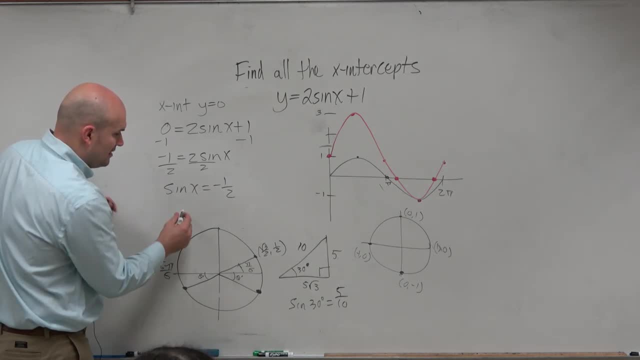 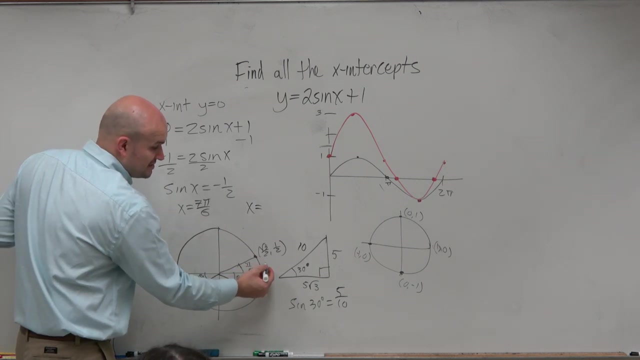 So, therefore, if I go in extra pi over 6,, x equals 7 pi over 6.. Right, OK, And then what else? And then this one: well, all the way around the circle is 12 pi over 6, or 2 pi, right. 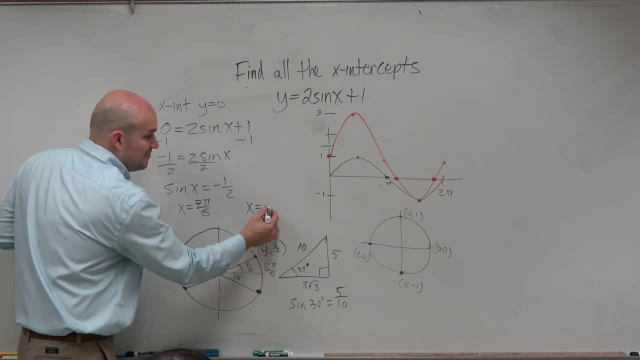 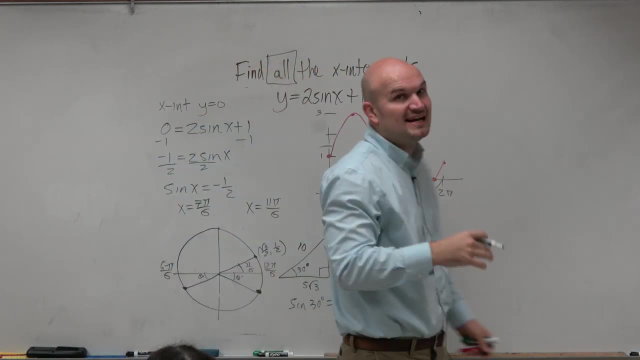 And so if I'm pi over 6 short, then that is 11 pi over 6.. But then the problem comes in, guys, It says, find all of the x-intercepts And what we just found is we just found the x-intercepts. 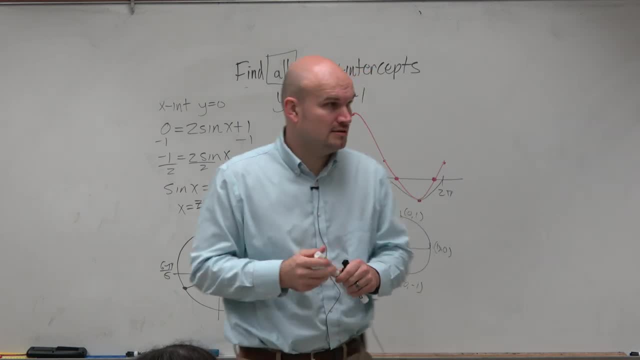 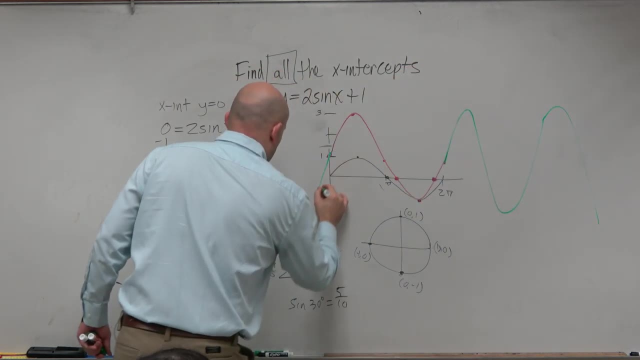 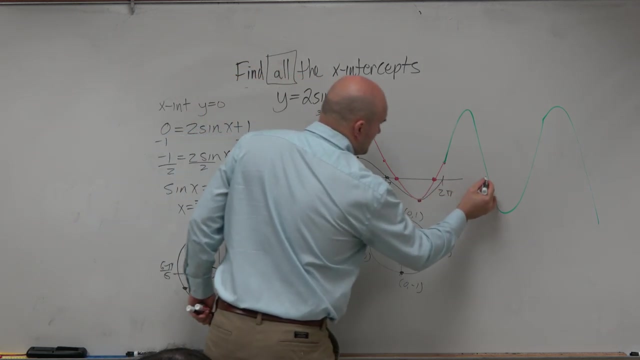 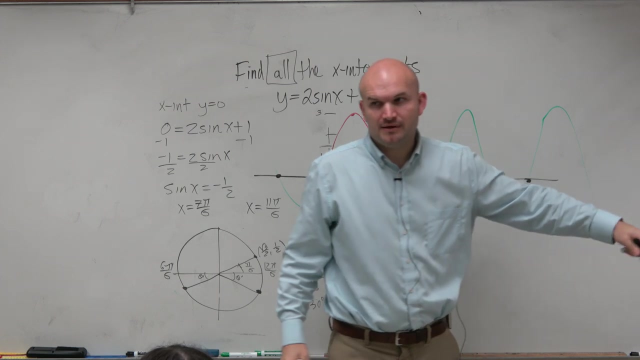 here. But we know that this graph does what Repeat, Repeats, So this graph is going to continue. So now we see that these intercepts keep on repeating. So now I'm going to think: well, how often do they repeat? 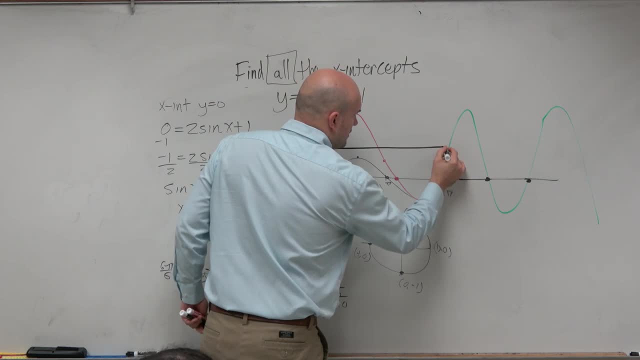 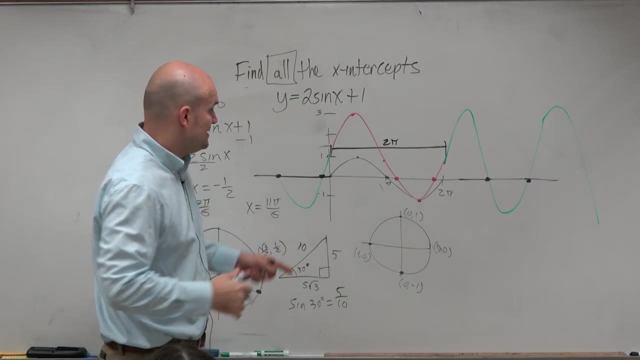 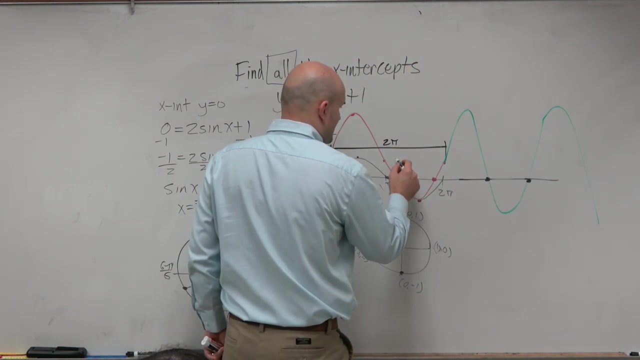 Well, I know that the period of this graph- because there's no change inside the function, the period- is 2 pi, Correct. So that means every intercept, every interval should also repeat 2 pi. So I mean my graph's not going to be perfect. 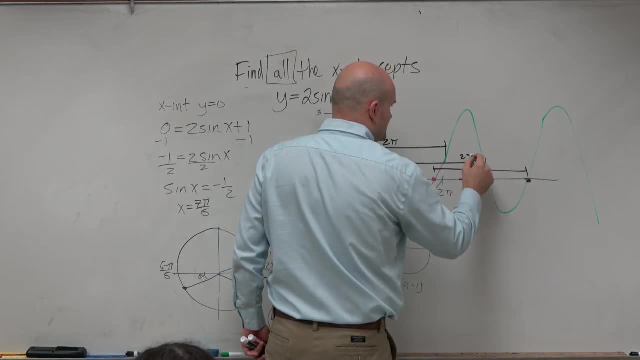 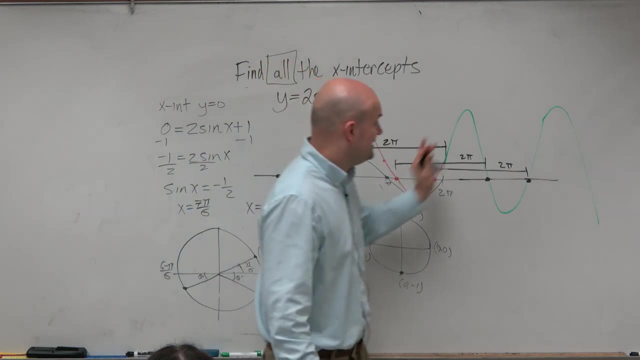 But do you guys see how those each look roughly like they're going to be at 2 pi. So if I need to represent this, because I could keep on adding 2 pi, I could also keep on subtracting 2 pi. 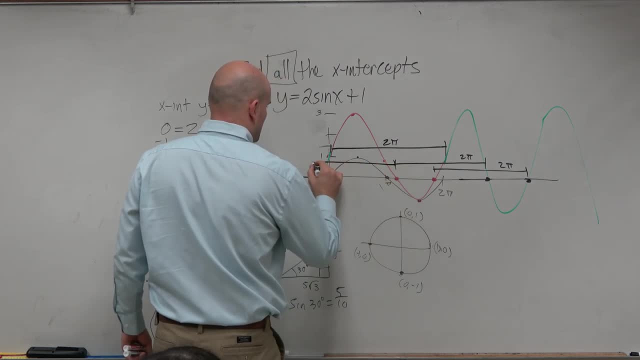 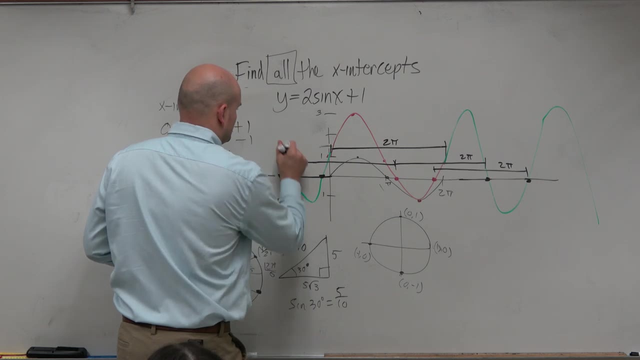 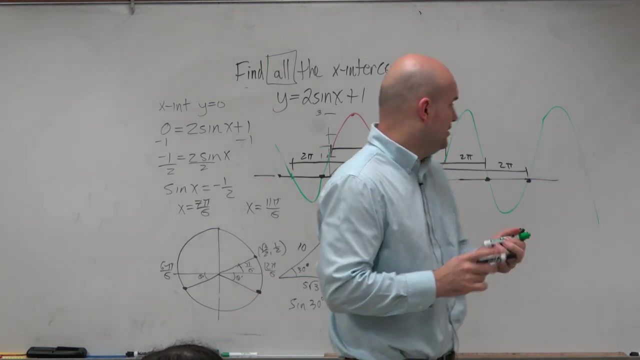 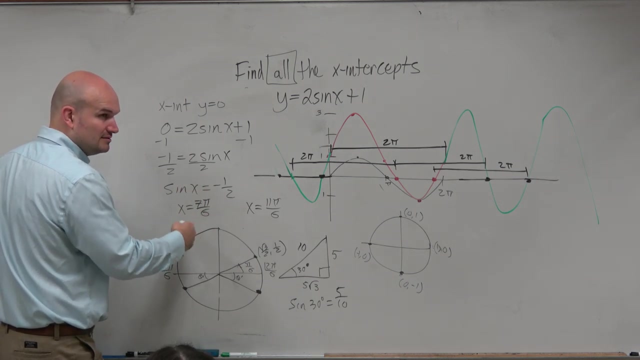 And that one. let's bounce that to you, Let's get that a little bit closer. So now we need to go back to kind of what we talked about with asymptotes and say, well, how do we write that relationship? How do we write 7 pi over 6 plus 2 pi, infinite, many times? 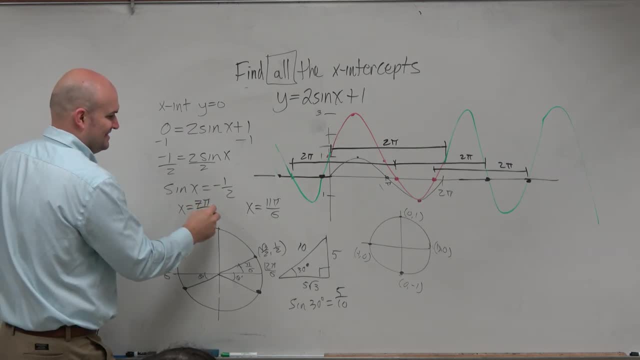 We can write that as Plus 2 pi n, Plus 2 pi n, And then this is plus 2 pi n, where again n could be a positive or a negative integer, And again we can look at the unit circle here, guys. 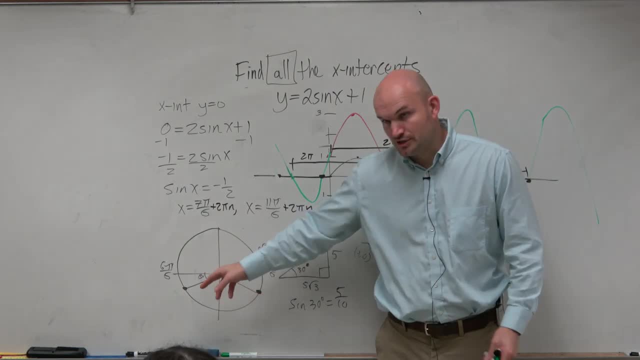 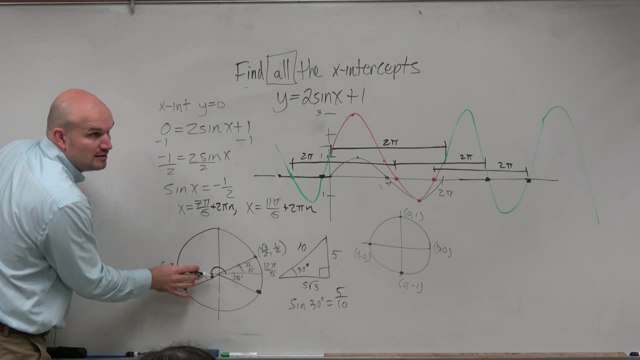 This is not a solution, right? So here is your solution. So here is 7 pi over 6.. If I want to get back to this spot, if I add 2 pi, I just found a what, What do we call those angles? 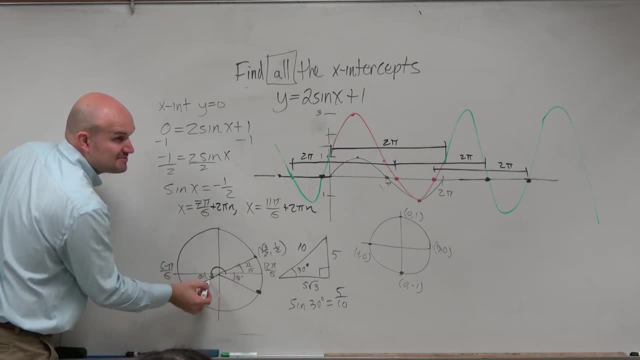 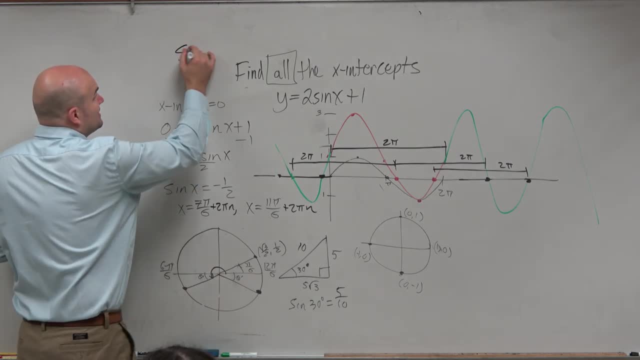 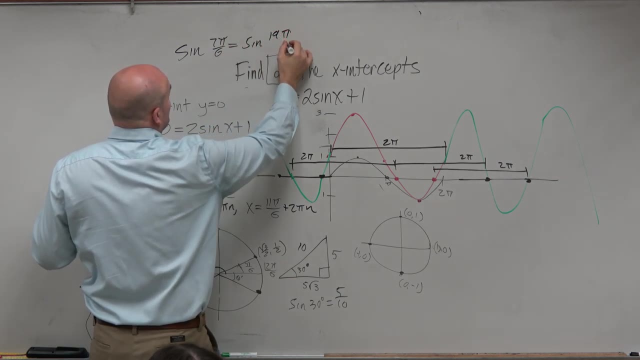 Keeps on taking me back to the same solution. Wouldn't you guys agree that the sine of 7 pi over 6 is equivalent to the sine of 19 pi over 6? They're the same value, right? They're just coterminal angles. 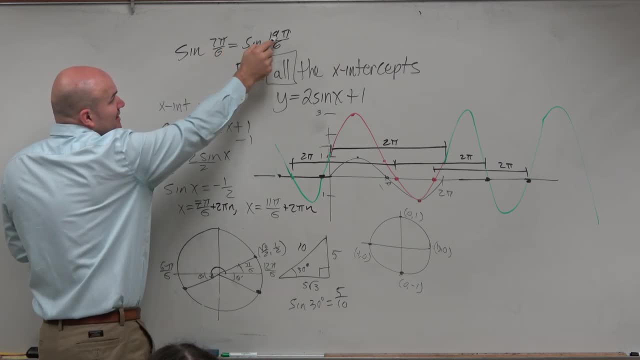 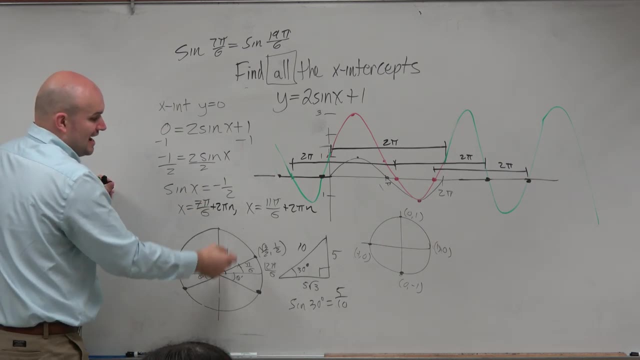 I just added 2 pi to 7, pi over 6, to give me 19 pi over 6.. They still end at the same terminal side, Their sine coordinate, the sine of that, is still negative 1 half. And not only do you have to add, you could also subtract.